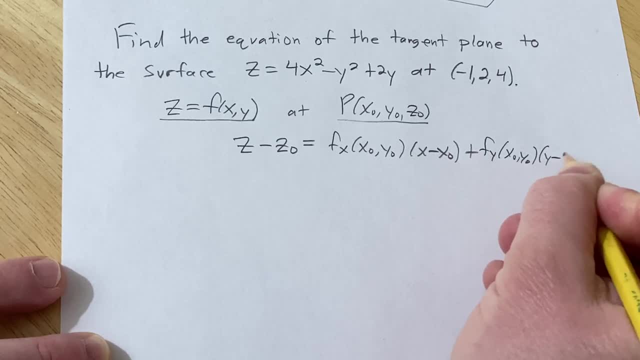 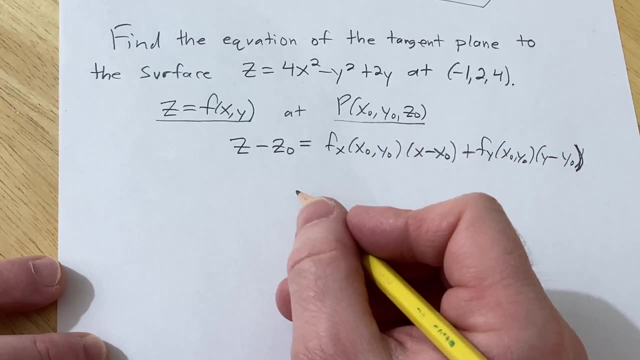 y at x naught, y naught times y minus y naught. And this is actually really simple. It's not hard. It just looks complicated but it's just partial derivatives And plugging in some numbers. it's not, it's not super tough. So in our particular problem, 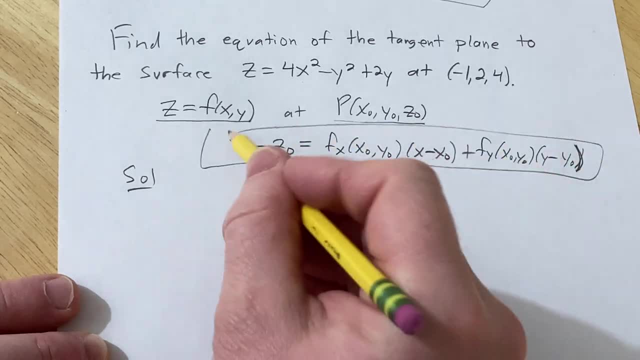 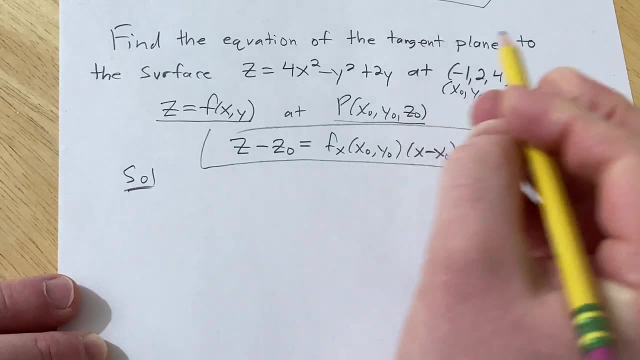 so this is the formula we're going to use. We have to compute the partials right. We have we've already got x naught, y naught and z naught, So let's find the partial. This is f, So you can. 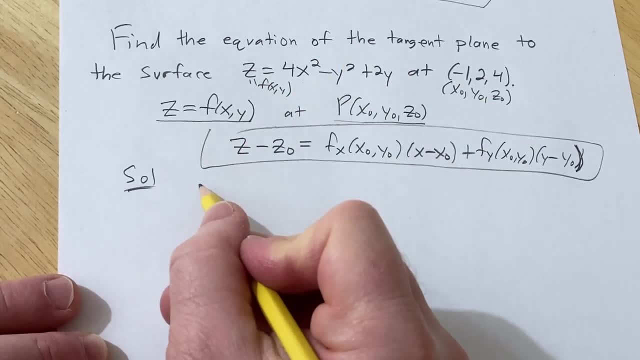 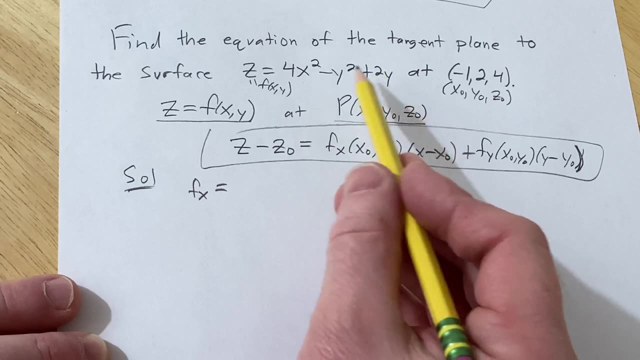 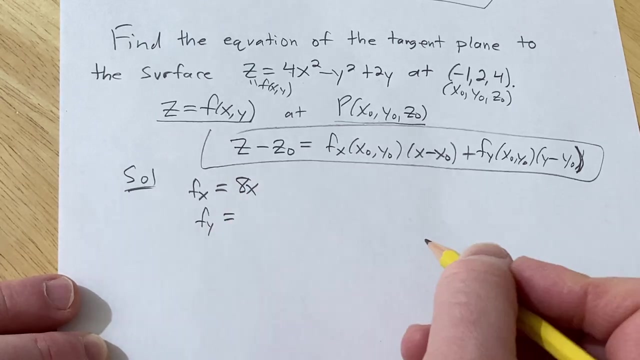 think of this as your f of x, y. So fx is the partial with respect to x, So all the y's are constants here when you compute this partial, So the partial is the partial with respect to x, So it'll just be 8x. So this is 8x. And then fy is the partial with respect to y. So in this case, 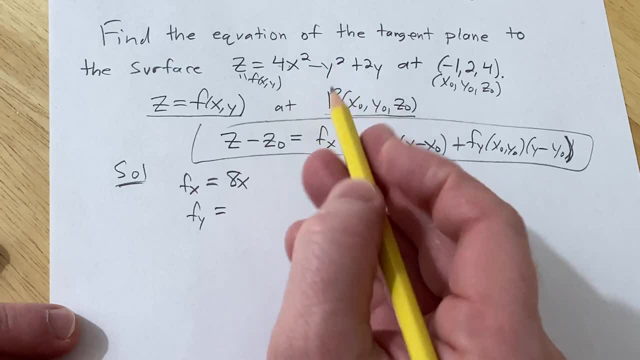 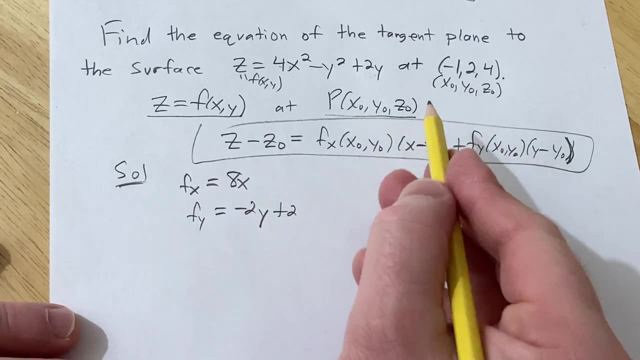 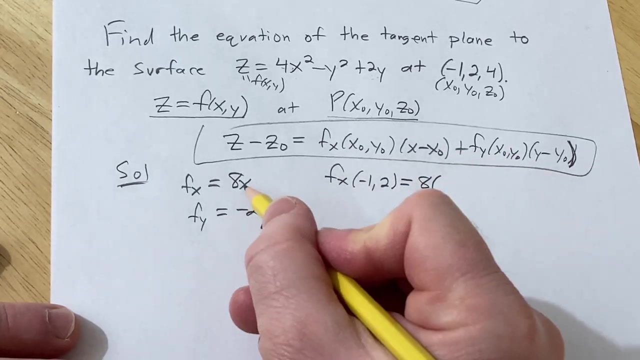 that's going to be 0 because all the other variables were constants. So it'll be minus 2y plus 2 because the derivative of y is 1.. Now we want to evaluate these at negative 1 comma 2.. So fx at negative 1 comma 2 is 8 times x is negative 1.. So it'll be. 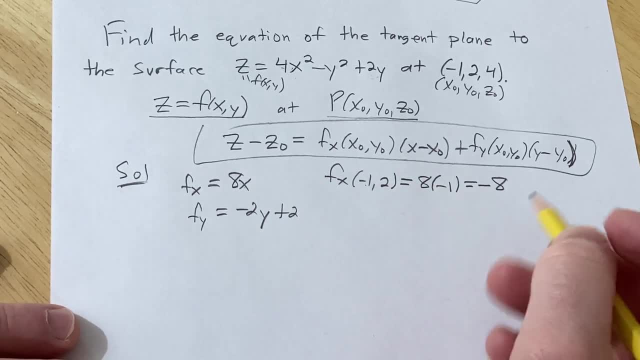 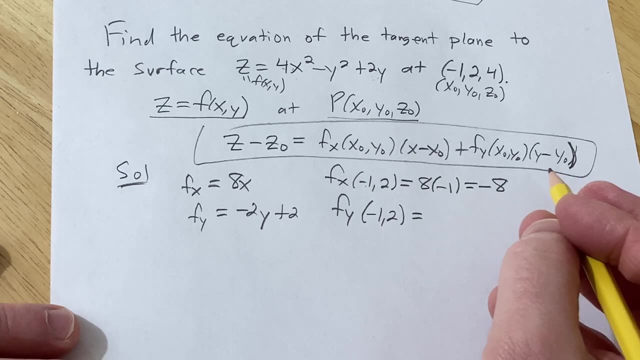 negative 1.. So negative 8 f y at negative 1 comma 2.. Okay, that's also going to be pretty straightforward, because it'll be negative 2.. And then the y is 2. So it's 2 plus 2.. 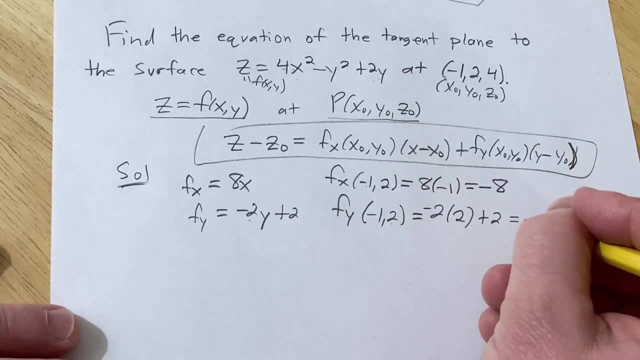 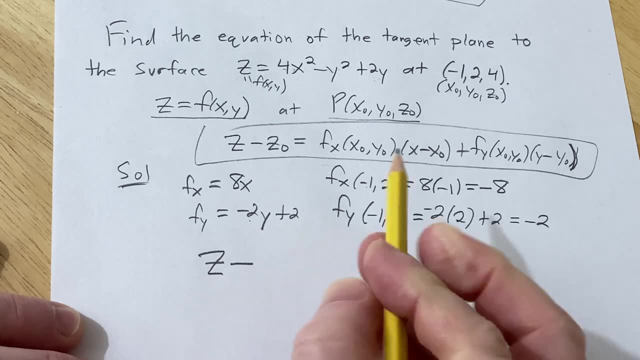 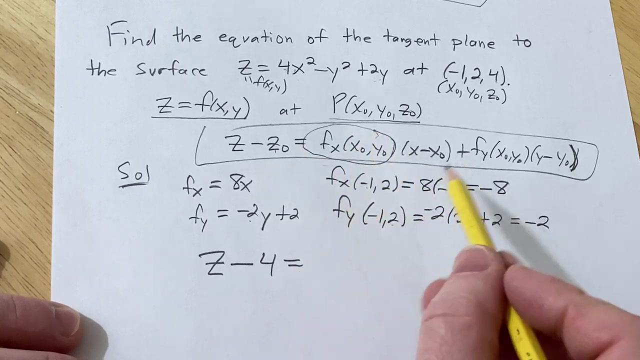 There's a negative there, So negative 4 plus 2 is negative 2.. Okay, so now we're just going to use the, the formula. So it'll be minus z, naught, which is 4, okay, so 4, equals this here. okay, which we have worked out right here. 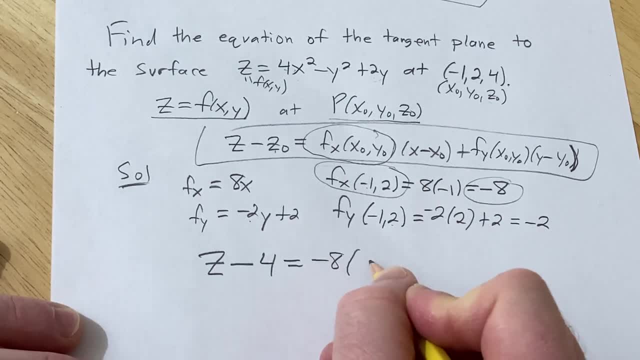 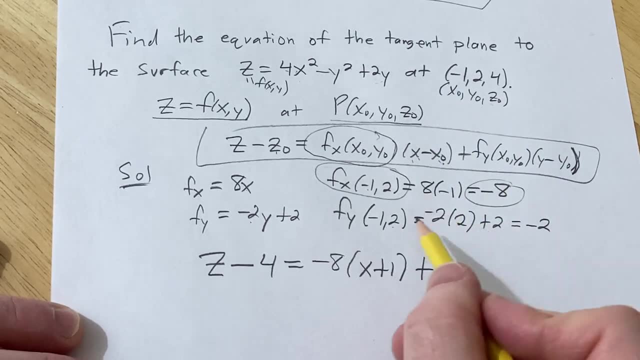 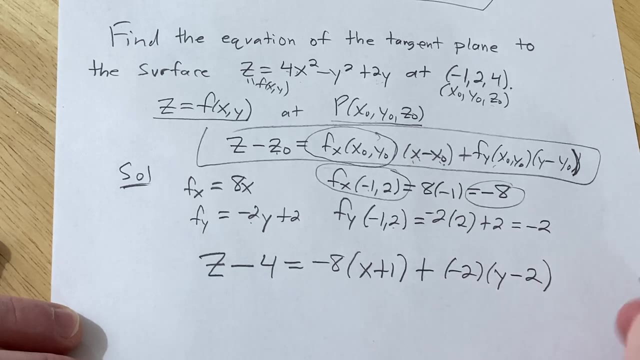 it's negative 8,, parentheses x minus x naught, but that's positive 1, plus. and then this one here which is negative 2, so plus negative 2, and then y minus y naught, so y minus 2,. pretty straightforward, right? so again, let's just check this. this is our negative. 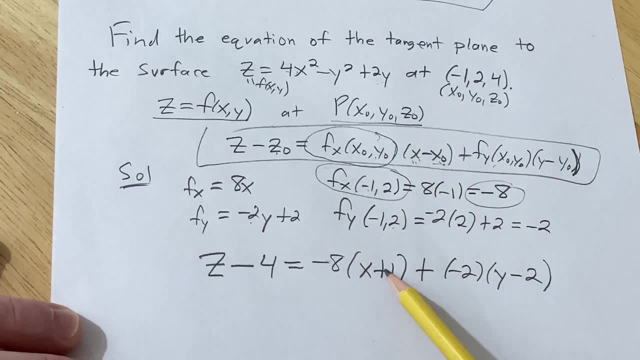 8, x minus x naught is x plus 1, because it's double negative plus this one here is negative 2, y minus y naught, so y minus 2,. the last thing to do, maybe, is just clean it up and see what.